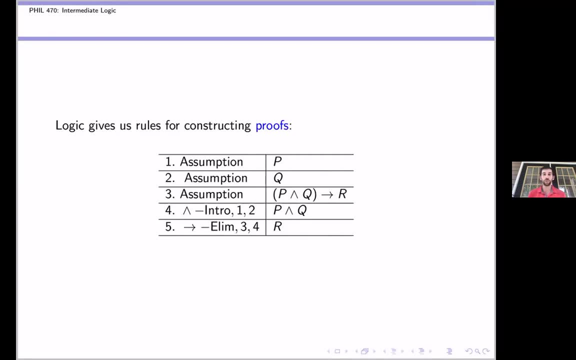 a derivation of the conclusion from the premises, employing only certain allowed logical rules. This kind of method is sometimes called syntactic. But are the things that we can prove guaranteed to be true, And can we assume that everything that's true can be proven? 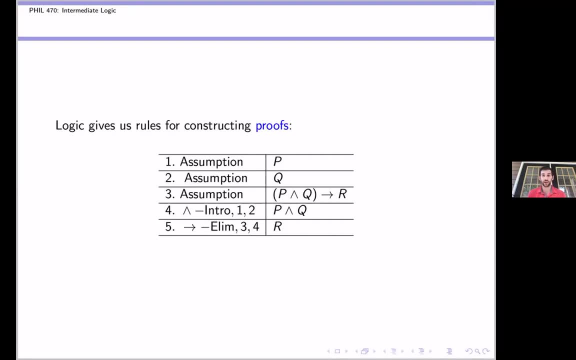 In other words, do we know that the syntax and semantics of logic are related in the right way? The central result that we'll establish in PHIL 470, the so-called soundness and completeness theorems, give a positive answer to these questions. 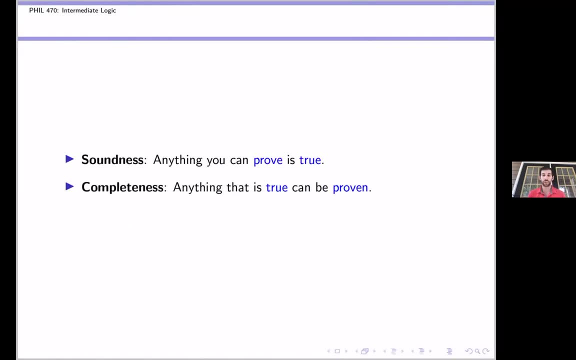 They show that logical syntax and logical semantics mesh together in the right way. The soundness theorem shows that anything that we can prove must be true, And the completeness theorem shows that everything that is true can be proven with our logical rules. Now, to establish these results, we'll need to learn new methods for proving things. 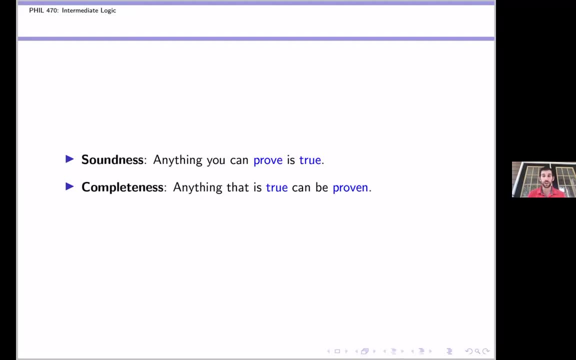 We'll learn about proof techniques involving mathematical induction and recursion. These allow us to prove things about the infinite, including infinite numbers and infinite lists of sentences. Our work in PHIL 470 will also lead to some very counterintuitive consequences, For example. 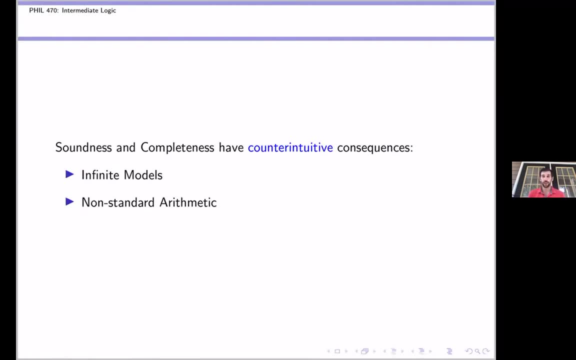 it'll follow that some simple mathematical theories, if they're formalized in a logical language, are much wackier than they first appear. For example, we'll look at the theory of the natural numbers, theory of arithmetic, which we can formalize with a very short list of axioms. 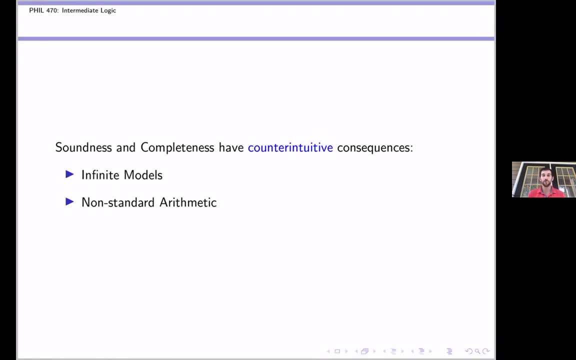 We'll be able to show that there are what are called non-standard models of arithmetic, non-standard models of the natural numbers, That is, there are systems of numbers that look very, very different from the ordinary natural numbers, but somehow they yield all the same truths. 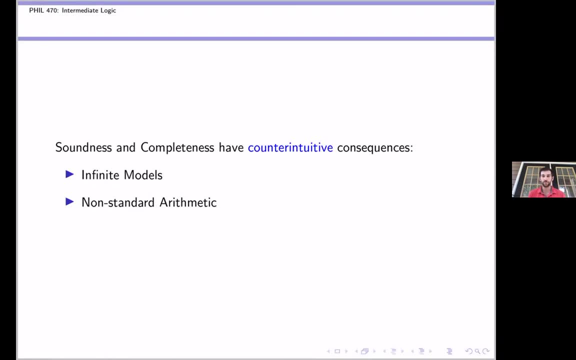 They have all the same things that can be proven within them, And that's just one example of something, one of the very interesting payoffs that we'll get from all of the work that we put in. So I hope that some of you will join me for next quarter for a journey into meta-logic. 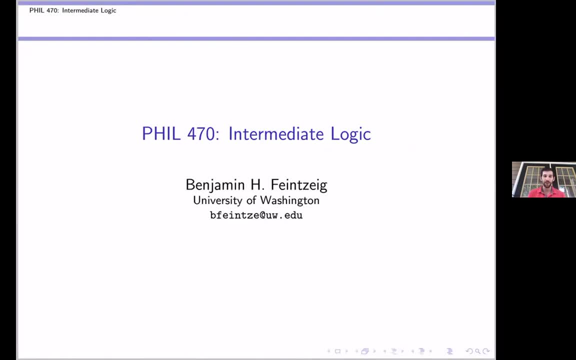 where we'll establish some facts about logic that are intuitive and some that are somewhat more bizarre.